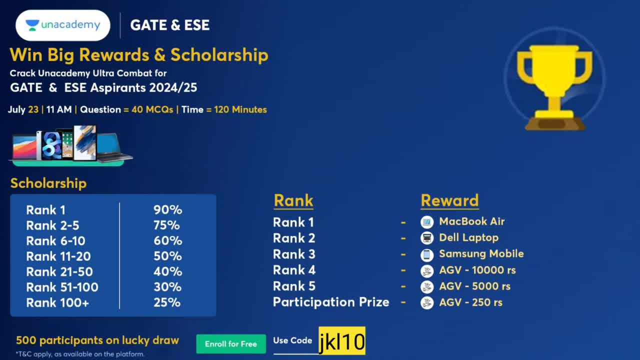 get up to 90% scholarship and many rewards such as MacBook, Dell laptops, Samsung phones and many more. And this ultra combat for GATE and ESC parent would be conducted on 23rd of July and the time is 11 am. How many questions you will get? 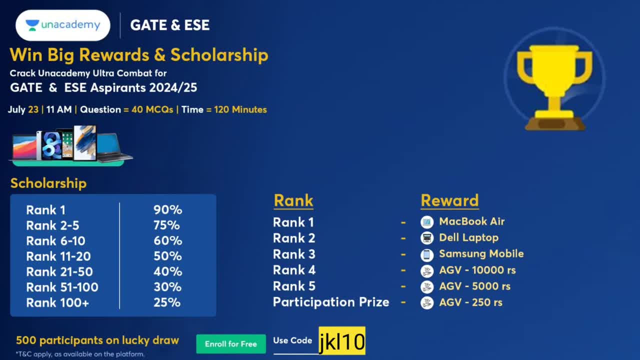 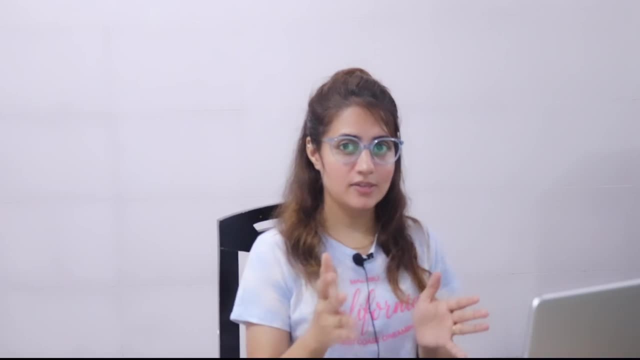 40 questions. MCQs would be there in this test and the time limit is 120 minutes. you will get to solve the questions Now. what is the syllabus? The syllabus will be general aptitude, engineering, mathematics and technical, And the most important thing is you can enroll for this test for this. 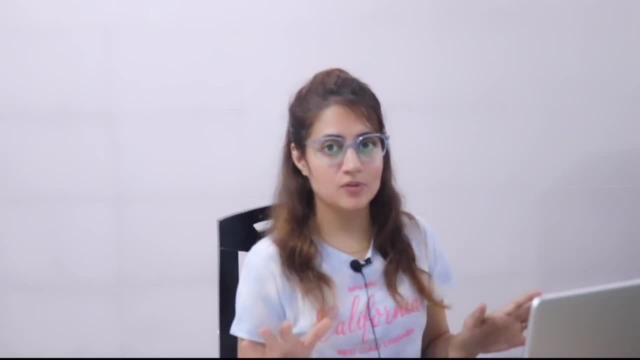 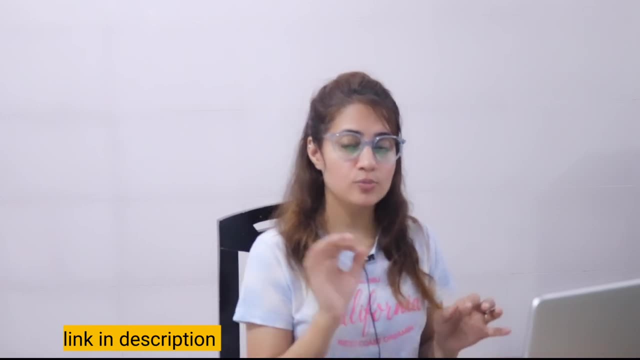 combat for free. You don't need to pay anything, no registration fee, nothing, right? So do not miss this opportunity and enroll today The link I'll put in the description box of this video and you can use my code, JKL, to enter the test. Thank you so much for watching. See you in the next video. 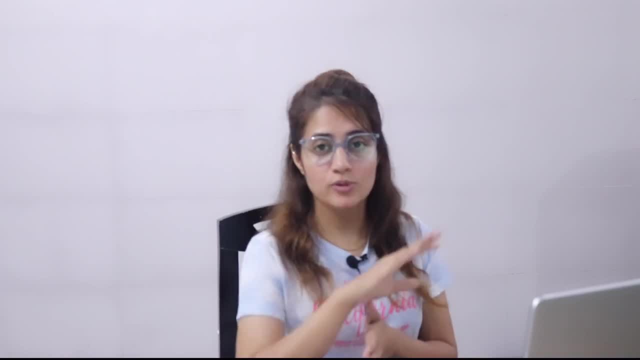 JKL tend to enroll for free in this combat right. So all the relevant information and link you will get in the description box of this video. You can go and check out. Okay, Now let's try to find out the answer of this question: Why, basically, we need OOP. 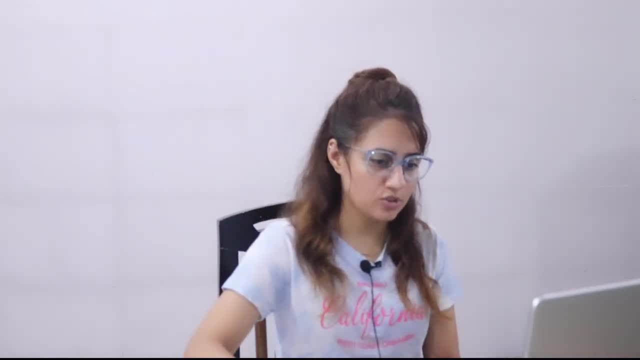 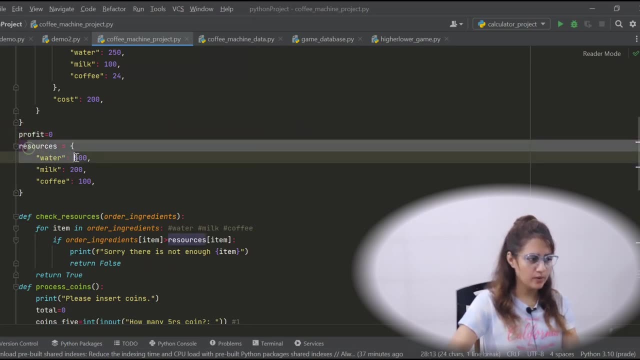 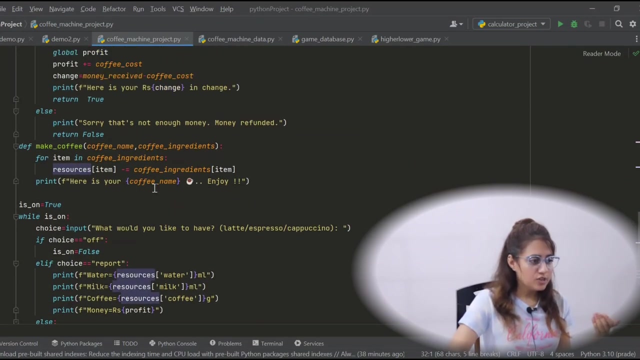 First see in the previous video. we have done this project, the coffee machine project, So this was our project. the menu resources: profit is a variable that is global. resources, also dictionary, having information that is global and we have defined many functions right and these functions are calling like: here we are. 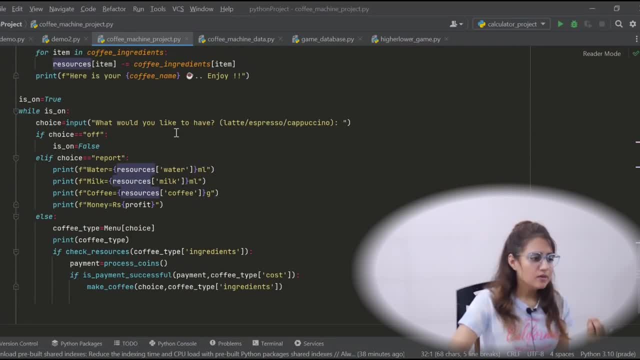 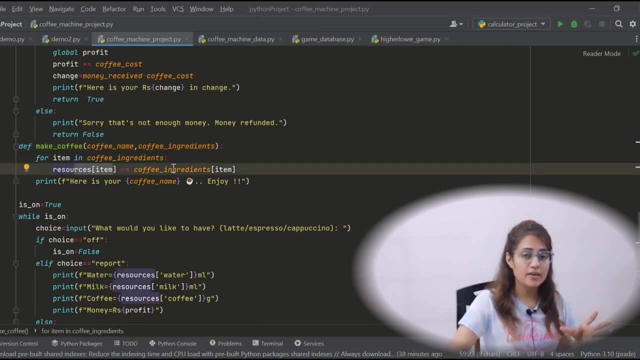 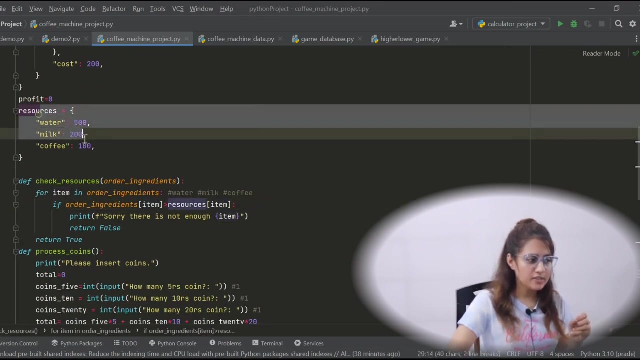 calling these functions and these are returning something and they are interlinked right. See, in this function we are in make of, in this function we are updating the resource item. resource item means these item because these are global right, and in this function also, we are accessing the resources because we are just comparing here. we are not updating. 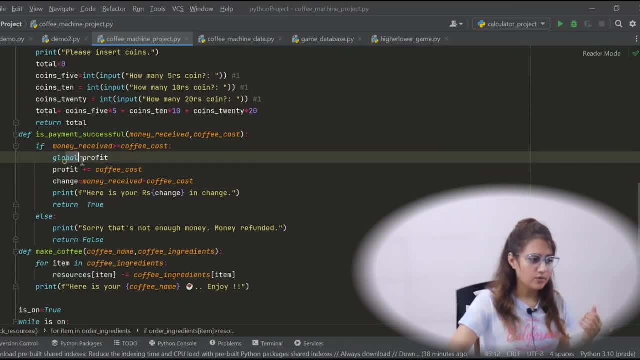 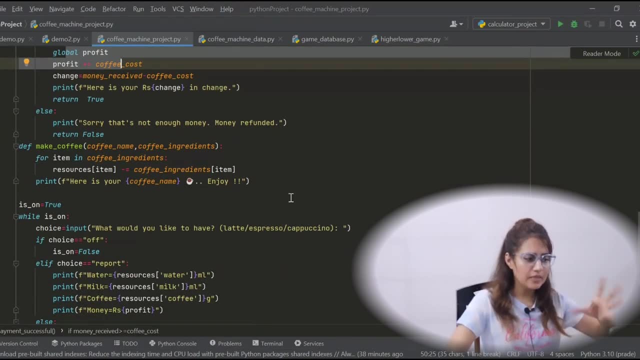 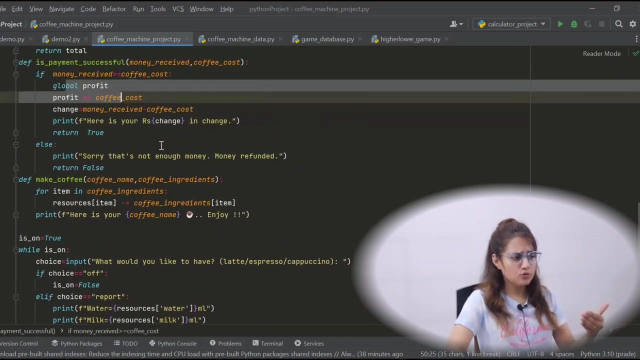 anything and in this, like we are we are, we are updating this profit, this global variable profit. we are updating this right. So these functions are interlinked with each other, having many relationship, right? Okay, now this approach is worked. here we are following the processor oriented program. 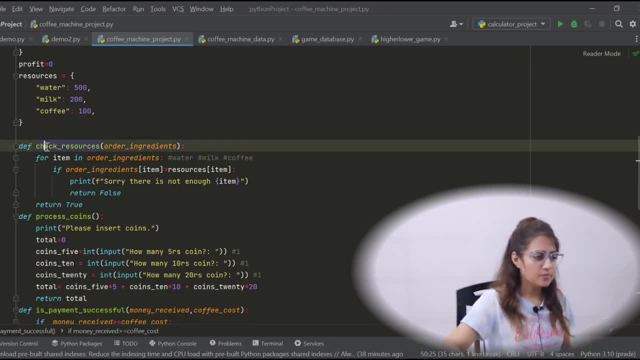 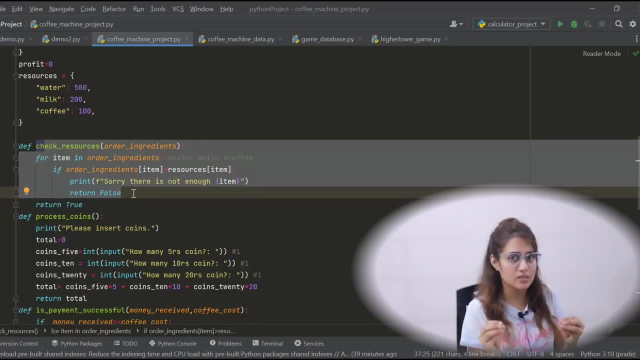 this approach, POP approach, right, Processor means these functions are known as processor means processor basically means the steps, how we are going to perform some task right and how we are going to perform this function, the check resources. these are obviously the statements or the task we 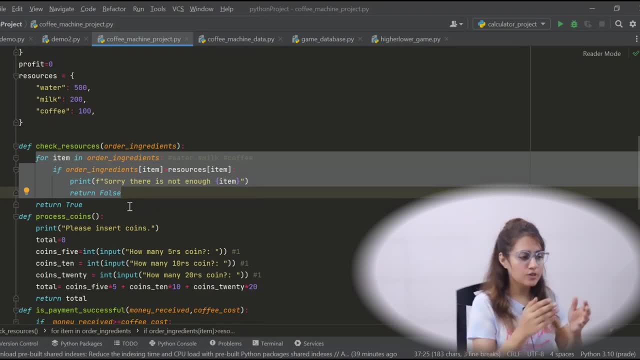 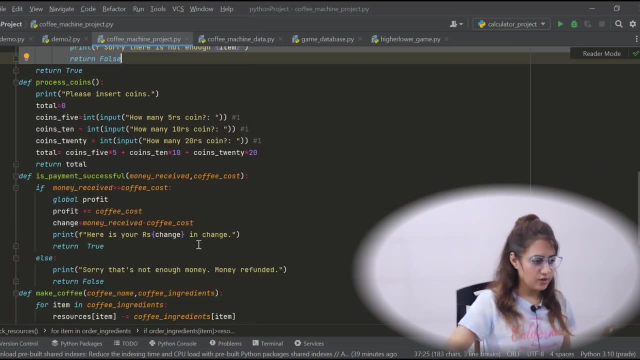 are writing the steps. we are writing, So these are what procedure, so we can say: function. so this is what POP approach right Now. yeah, that is fine, we are following POP approach. so why now we need OOP approach? because this is also fine, right. 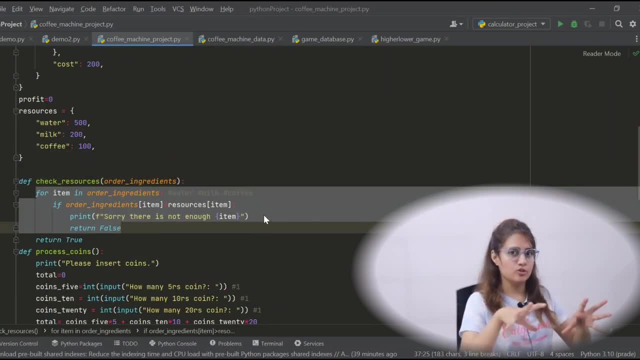 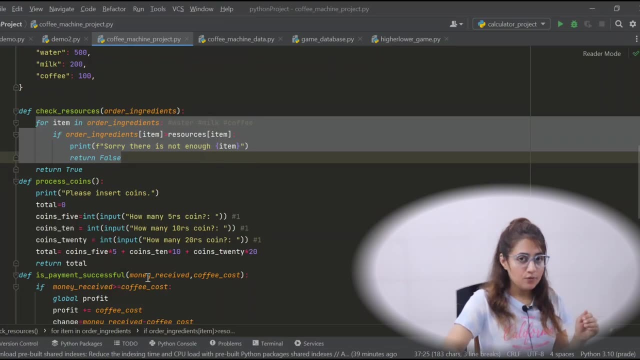 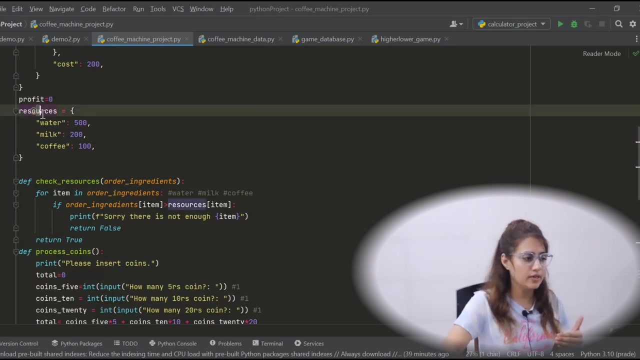 But in POP approach we can handle only small project because, see, it is just a simple one, coffee machine project. and here, see, we are having multiple functions and the main important thing is these functions are updating global variables. The profit is global, variable resources, this dictionary is also global, obviously. 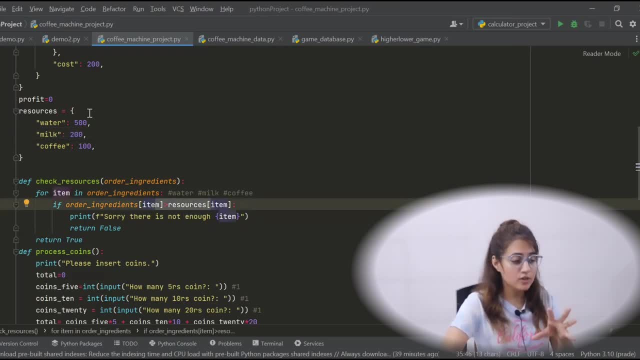 So in many functions- more than one function- we are accessing this resource and one function is updating this resources, and in one function we are updating this profit right. So we are updating the global variable or the data. So suppose we are dealing with a large project, a large scale project. there we are having 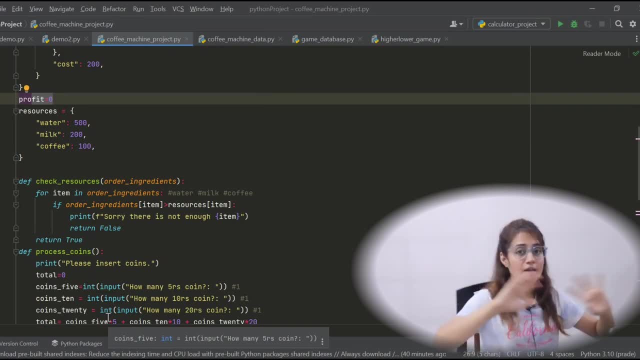 multiple functions, 50 functions or 100 functions and many global variables, right? So it would be very difficult for you guys to track, like, which function is accessing which global variable, which function is you know updating which global variable? and, accidentally, if we update a global variable? 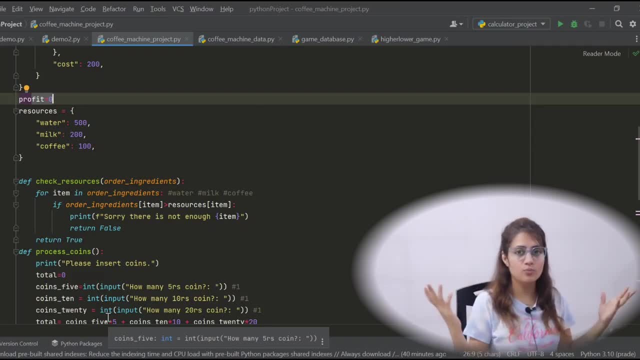 If we update multiple global data in any function then maybe it will give us some error or some unusual you know result right, some unexpected output right. So main thing is- I think now you have noticed- main thing we are focusing in this approach, POP approach- on functions- how to do the task, the functions, the procedures- not on data. 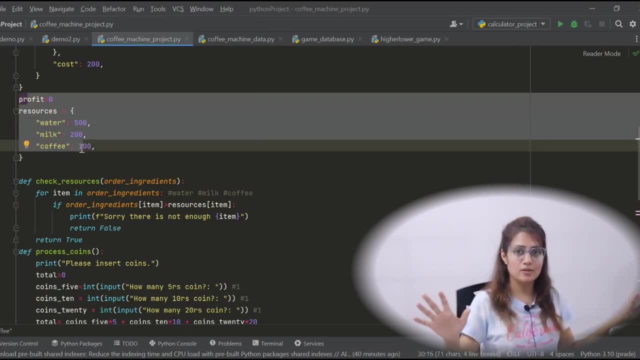 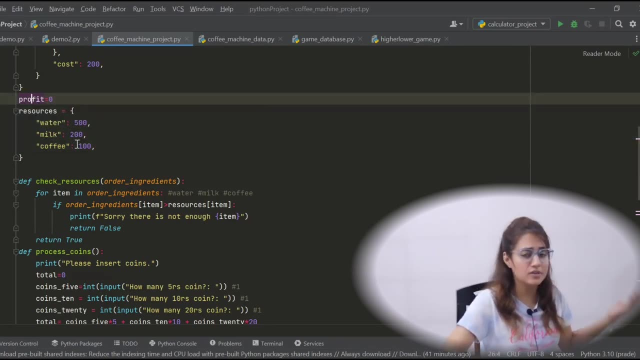 Data is now. Data here is freely moving during the whole program because obviously the global data is moving freely. Any function can access this data, any function can update this data. right, It means there is no data security. data is freely moving. we are just focusing on the 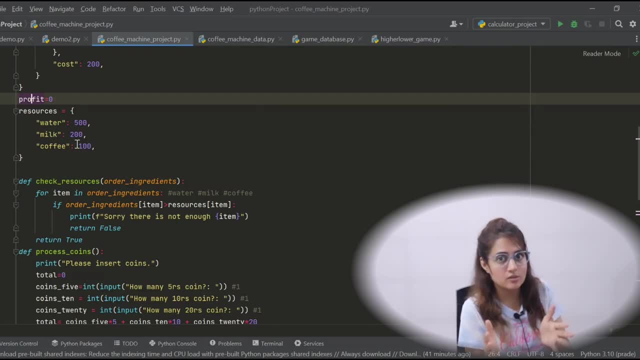 procedures or the function or means you can say how to do the task. On this we are focusing more. So one drawback of this is what? Data security? I hope you got Why I am saying the data security, Data security. There is no data security in POP approach. 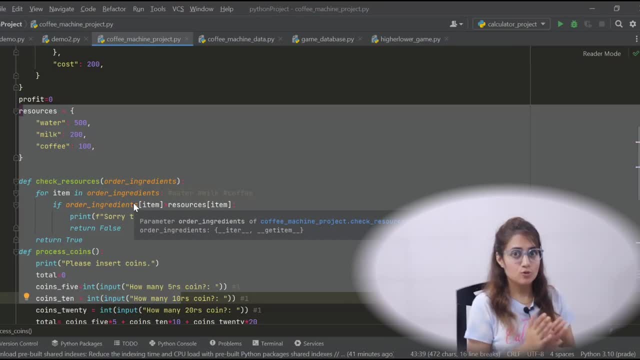 I hope you got this thing now right with the help of this example. So now, if you want to handle any real world problem, any large project right, then definitely it would be not easy to manage that project, to implement that project with the help of 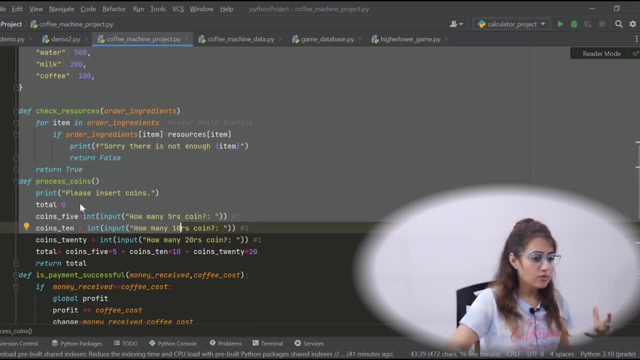 this POP approach right, because of the complexity and the relationship between those functions and all: How to manage the relationship, how to check which function is, how to track which function is using which global data and which function is updating which data, and all right. 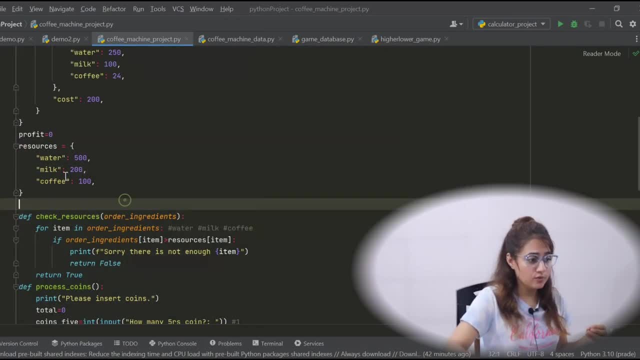 Because we are not focusing on data more and if suppose, if maybe you think like we can do, we will take like no global data is there. we just change this type of this global data. just take local data. So all the functions which are accessing that global data, you have to do accordingly. the 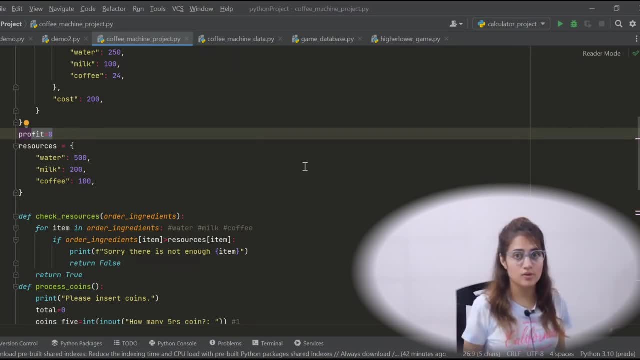 changes in those functions as well. We have to resolve those functions as well, right, because maybe many functions are using that global data, right, Okay, So because of the complexity and the number of relationship are very complex here, it would be very difficult to manage that thing with the help of this POP approach. right, and obviously. 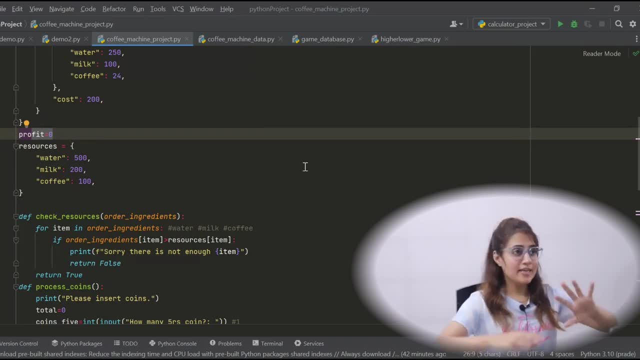 the data security is not there. and yeah, obviously, if you are implementing any real world project, then we know that the data is how much the data is important. like maybe I want like anybody can access my name, Jayanthi, but only few person can access my mobile number, not all the person. 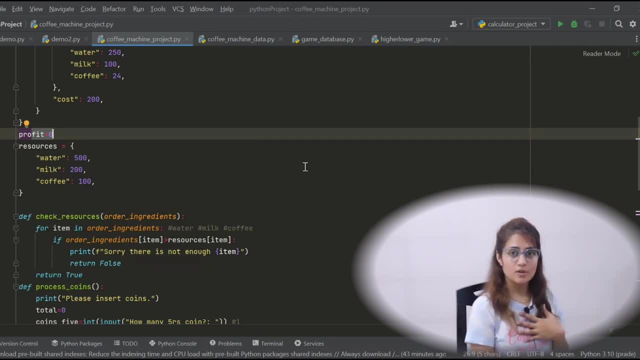 Obviously I want my data safe, Okay, Okay. So if you want to implement, if you want to model any real world problem, real world project, then definitely you have to focus on data security, and data security is not in POP. You cannot, you like, you cannot- implement data security. you cannot achieve data security. 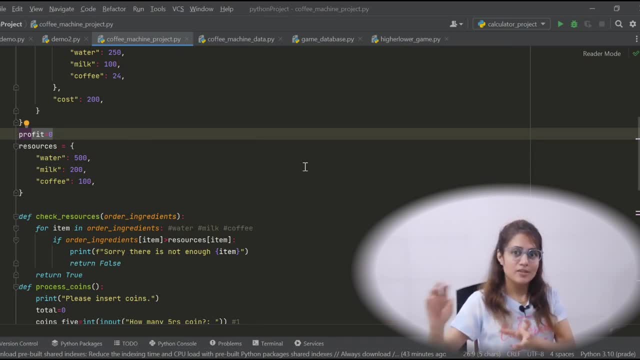 in POP approach. That is why we need another approach and that is in OOP. yes, we are having data security, and why that. I will tell you how you can implement data security in object oriented programming. There are other drawbacks also in this approach: POP approach, like there is no inheritance. 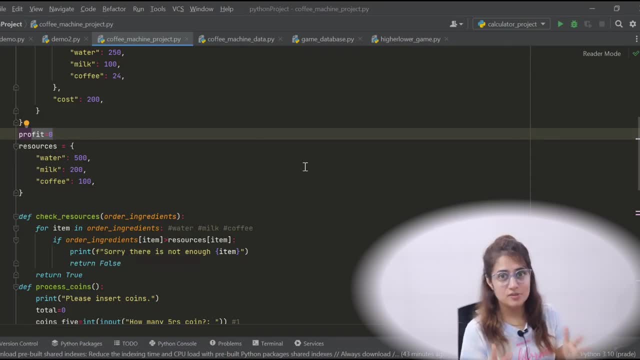 no virtual function, no operator overloading, no polymorphism, no data hiding. Many other things are there, but now I know you don't know about what is inheritance, what is data hiding, what is virtual function, what is polymorphism. So that is why it will not be. you know, it would not be easy for you to understand these. 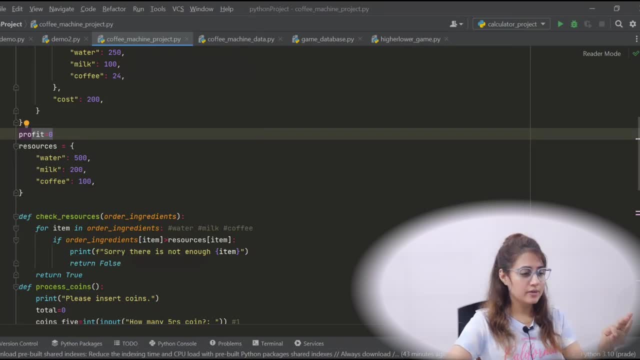 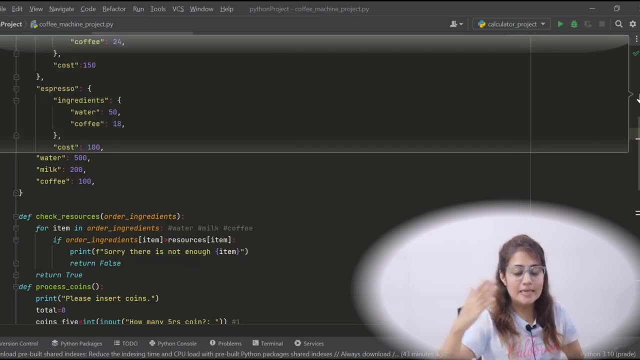 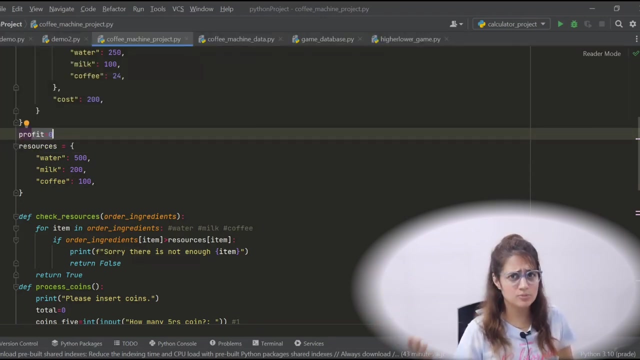 things right, but I am sure data security is one thing, one drawback: that you got exactly what is data security and why I am saying this right Same thing. in later videos we will discuss what is inheritance, what is like you can say that virtual function, and all. we will be discussing polymorphism, data obstruction. 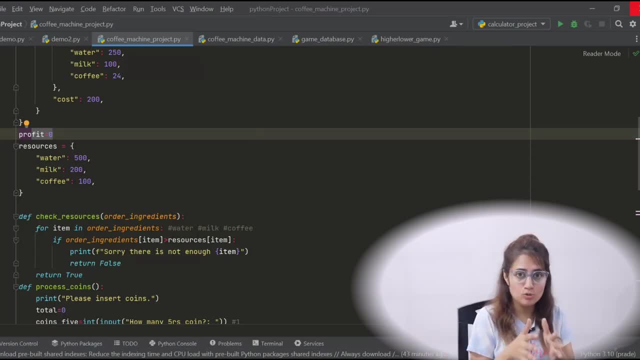 data hiding, then you will get why I am saying right now like POP is not having these things right. It's okay. if you are not getting anything of these terms, it's okay, it's normal right, because it's first lecture of OOP and definitely it would not be easy for you to understand. 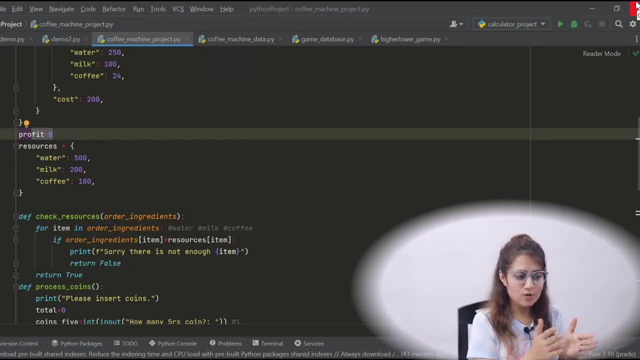 everything in one video, right, But till now I hope the data security was helpful. Thank you, Bye bye, Take care, Bye, bye, Bye, bye, Bye, bye. Now, object oriented programming is used to model now the real world projects. right Now, first thing we will see like what is object. 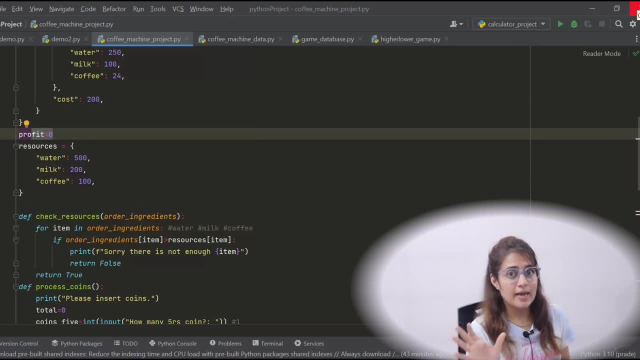 We know Python is object oriented programming and I think you have heard this line also. everything is considered as an object in Python, right? Why I am saying this? Let's see with the help of this example. See, if I take a variable like a is equal to 1.. 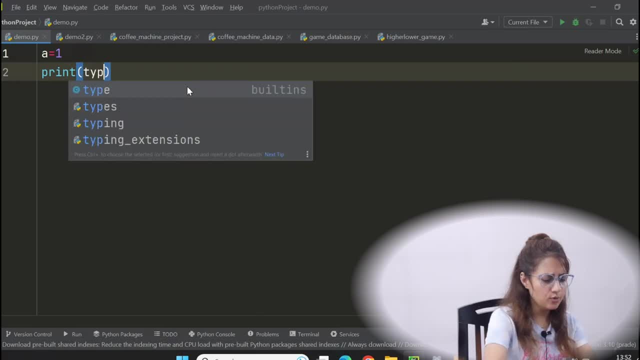 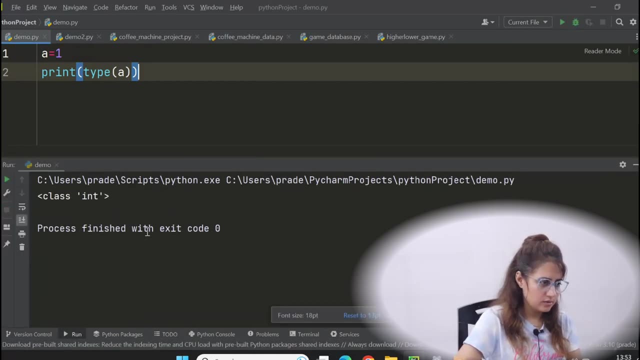 And if you print the variable a, you can print the variable a And you can print the variable a If you print the type of this variable a, then what you will get? Just focus on the answer. see class int class, because here we are having a class that is: 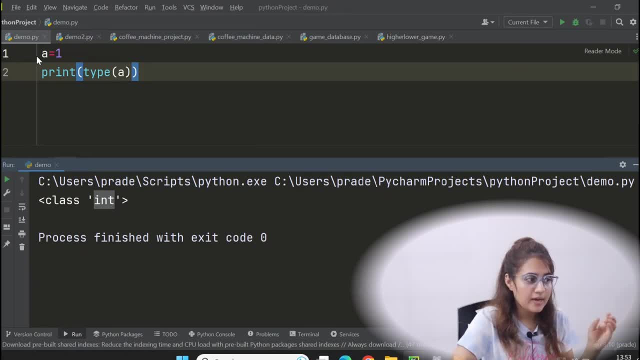 predefined in the library of python class is int and this a is what? It's? just an object of this class int. If I will not take this a, if I like want to find out the type of this string. hello, now let's run this. see class str. now, this hello is an object of class str. 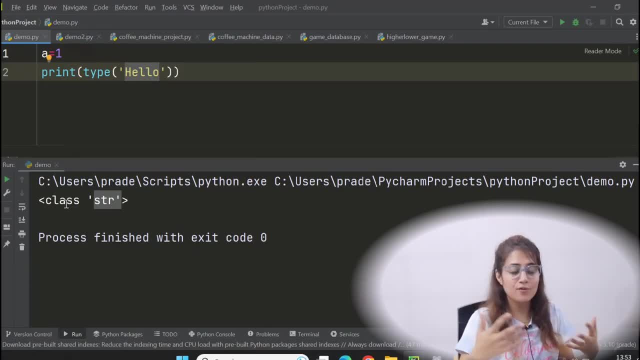 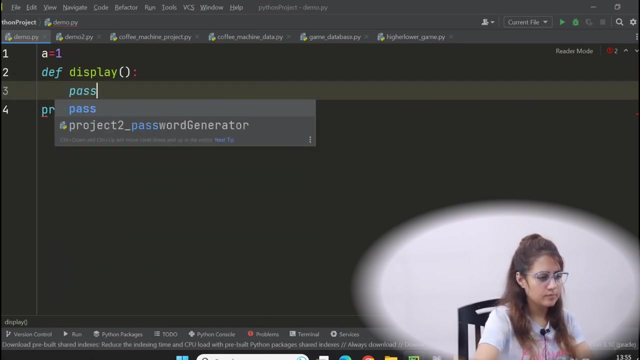 So this is built in class in python. that is why I am saying: everything you deal now this hello is what an object. this a is also an object. everything you deal is in python is what An object. Let's take if I have a function display, and there I am just using the past statement. 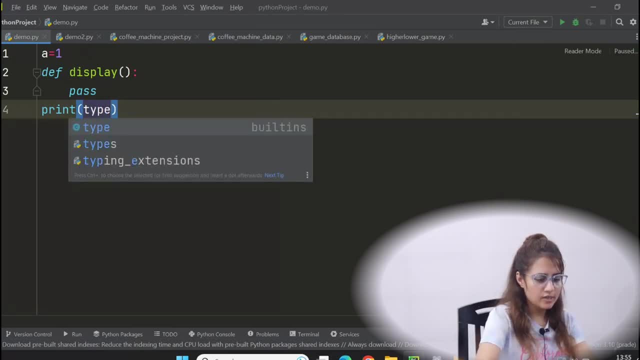 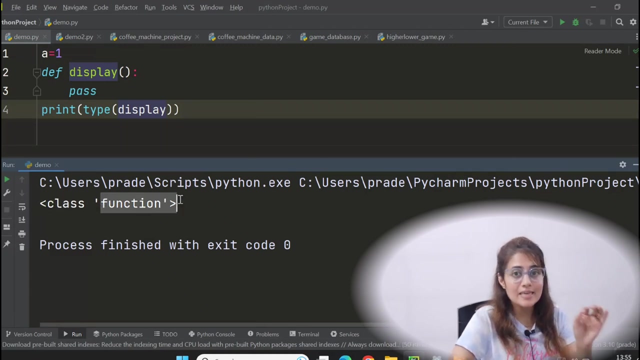 nothing I am going to write and I want to find out this type of this display function, this you need to write down name of this function: display. let's run this and see class function. so there is a class inbuilt class function and this function is an object. 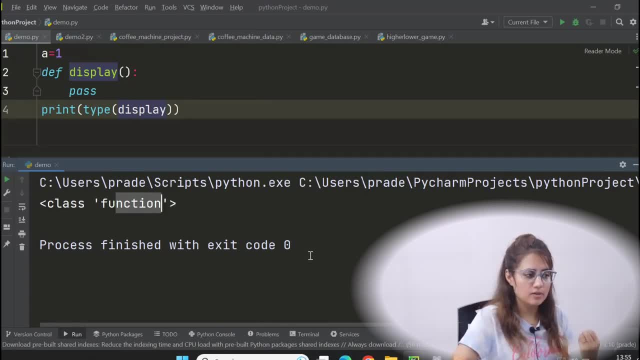 This is just an object of this class, this class. that is why I was. I was saying like everything in python, whether it's variable function or any string or not, everything is considered as object. now you got why we are saying like what is an object and why. 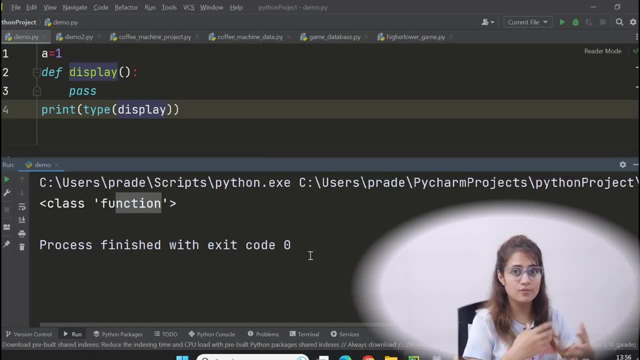 we are saying this, so you got this idea: inbuilt classes. we are having in python many inbuilt classes, right, and the object you can use, fine, and see, there is a class, str. see, you know this, hello is what? just, it's a string. if you want to find out type, so the 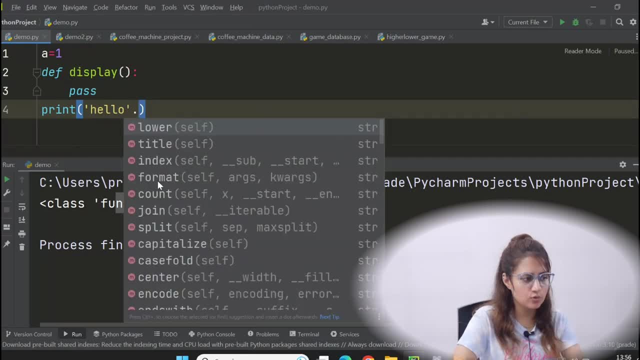 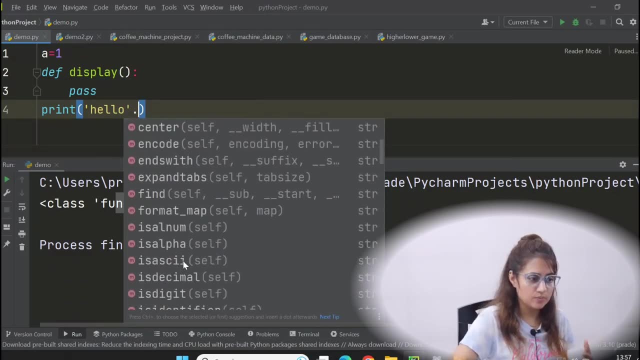 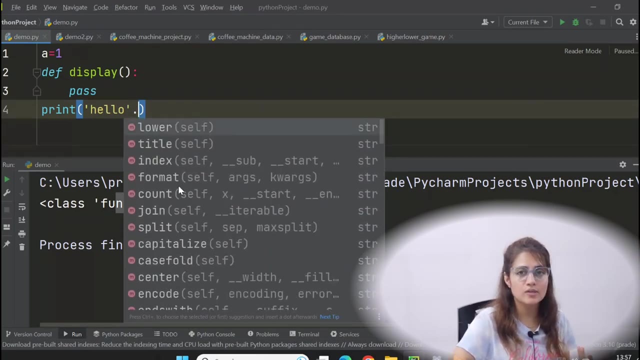 class will be string. so if I use something like hello dot, so the class str, that is having many functions, lower title index and many function, see right. so these functions you can use on this object because this object is of str class type, right? so if I use this, 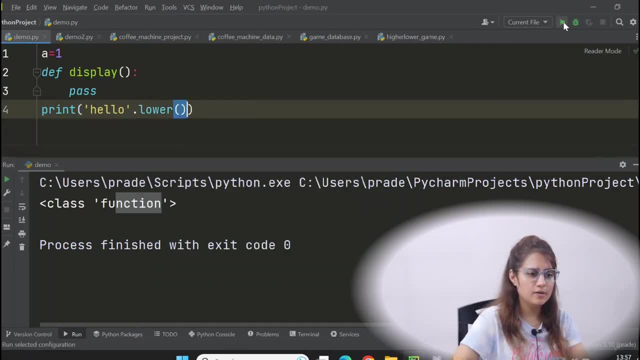 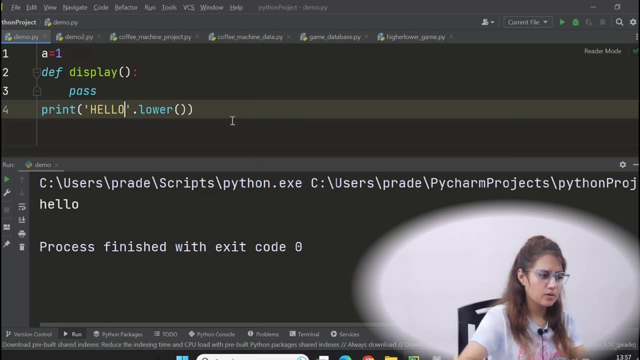 dot lower and if I print, if I run this, see this is already in lower, so it would be. let's suppose I will do this in capital letter and see it will print in small letter, capital letter, but dot lower means small letter. so there are many inbuilt function, also that 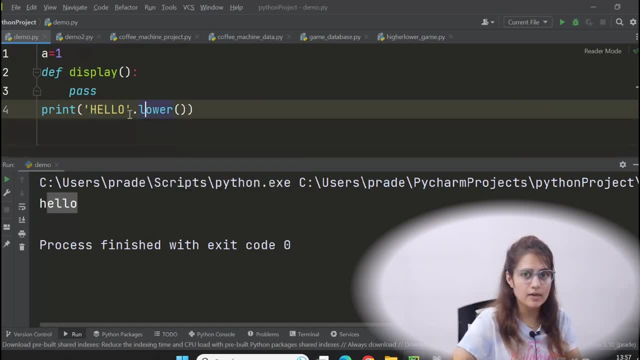 you can call on that object with the help of dot operator, right? what are the object dot, whatever the function, is there of that class? So many classes, and those classes are having inbuilt functions, those you can use on those object, right? so I guess you have some idea now. objects, and all right. 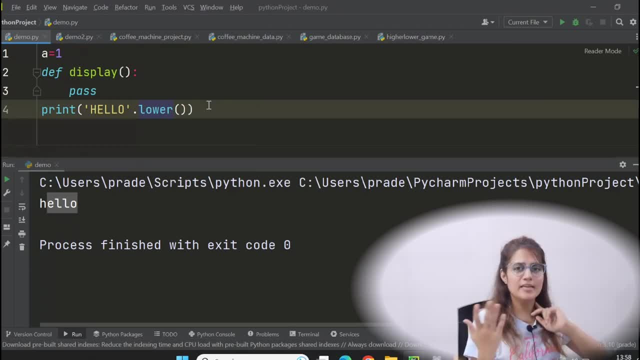 Now oriented. oriented means in simple English language if we say: then like it's interested in a particular thing or a particular person, so we are basically interested in object. that is why it is known as object oriented programming. so our interested or main focus is in on objects. 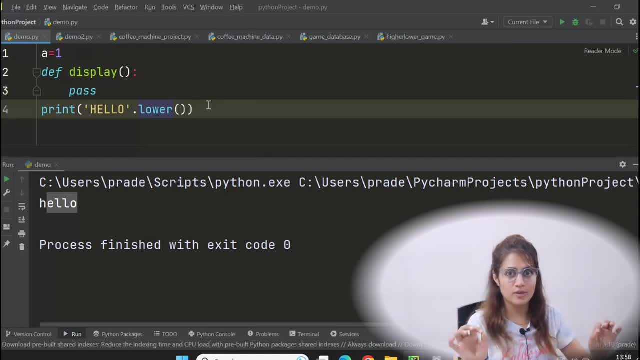 right. That is why it is known as OOP. like you know, this show up is male oriented, or female oriented means in this show up the product, all the product you will get are of males, not females: male oriented, female oriented like this. so, object oriented, we focus on. 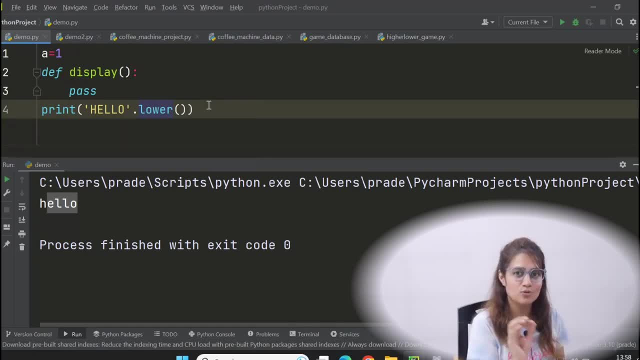 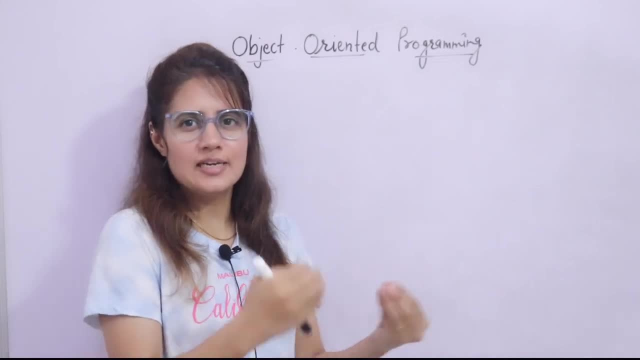 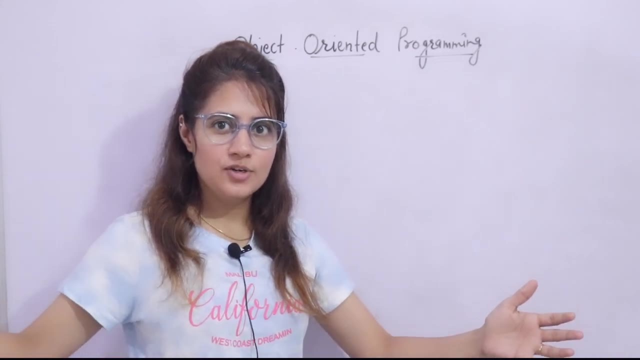 we are interested in objects. that is why it is known as object oriented programming, right? So I hope the answer of why, why we need OOP, that is somewhat clear to you guys, because we have done some. So what is the advantage of OOP? not all, because everything we will be discussing later- videos. 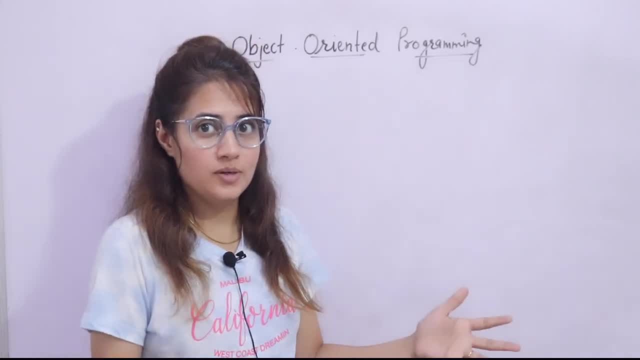 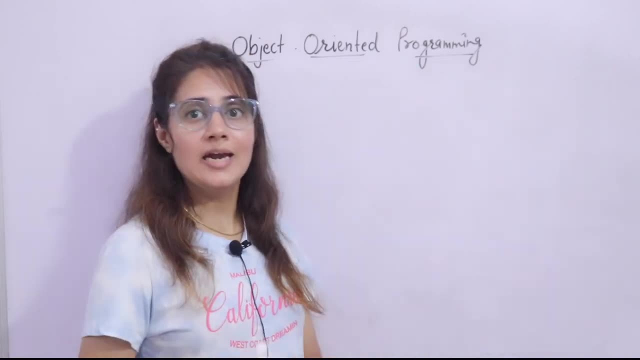 then you will get all the advantages and benefits of OOP. If you, you know, understand to a certain level what is OOP and what are the advantages, then definitely you will get why it is always better to use OOP and why in the industry. 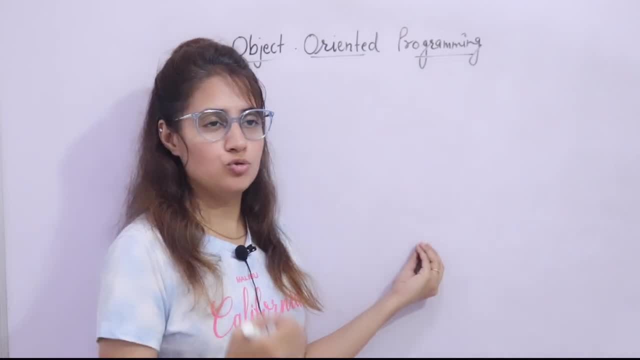 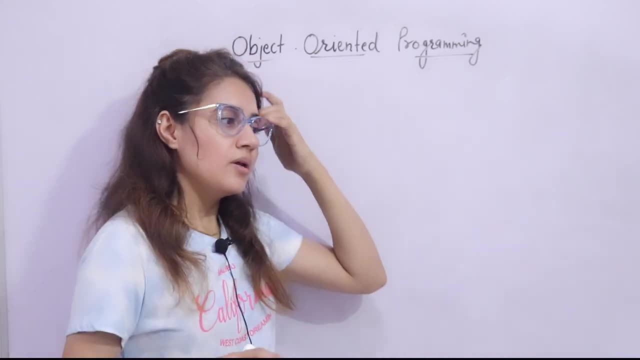 you know, in the companies they use this OOP approach to you know: implement project, large project, real world project, right Now. let's take a simple example. So let's say you have a project. Let's take a simple example. 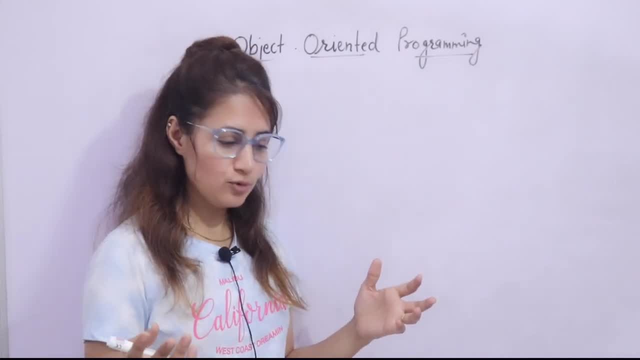 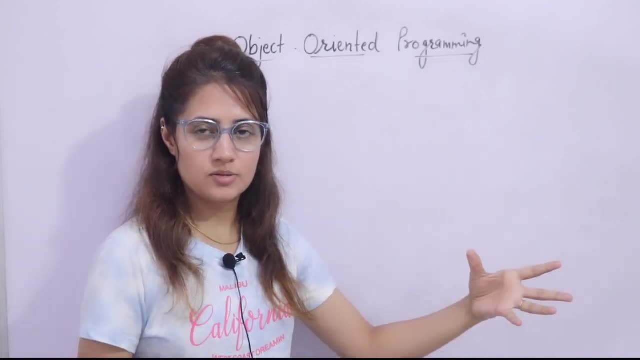 If real world problem I am taking if I am going to start a YouTube channel, right. So in starting I am the only one like one man arm so I can teach some subjects. I am the editor, I am thumbnail designer, I am the social media marketer, I am the instructor. 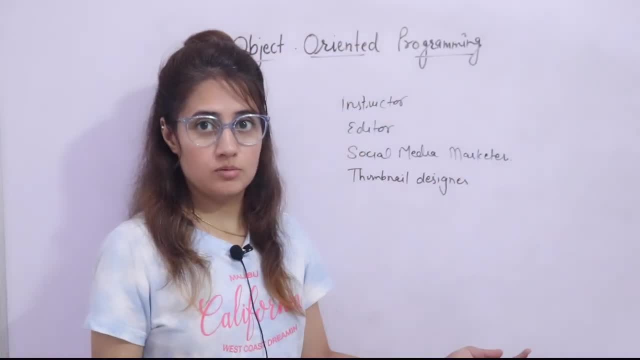 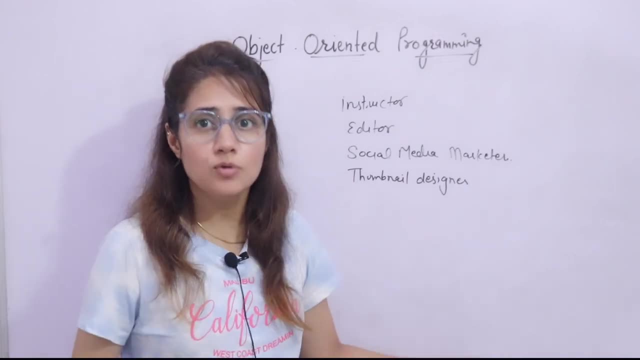 right, But I want to start many courses: C, C++, Java, computer network, DBMS, operating system, data structure, web development course and many more courses. Then definitely if I am a one man army, then it would be very difficult for me to manage. 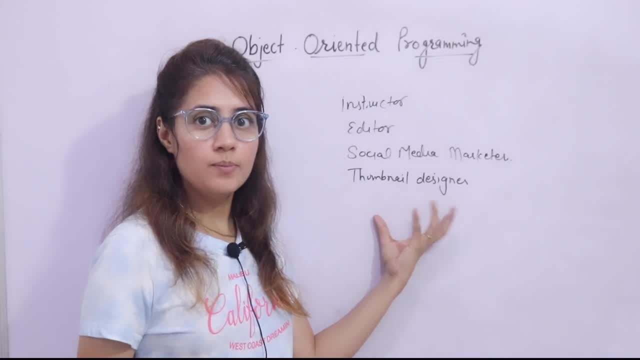 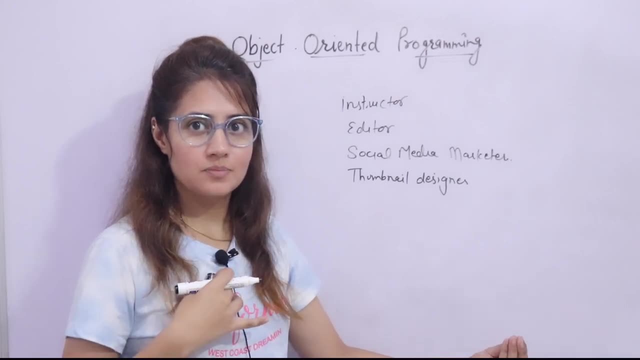 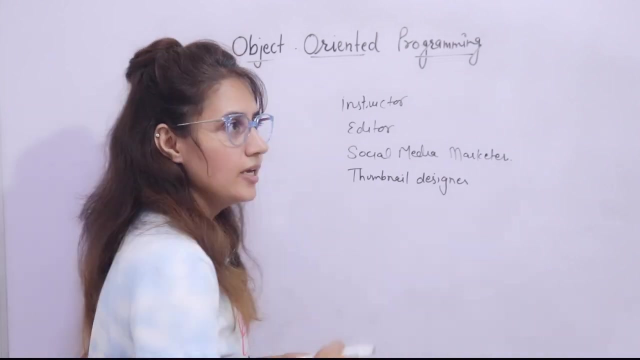 everything right, So this would become more complex. if you want to grow your YouTube channel. obviously You got it right for one person, fine, Now what I can do to solve my problem. I can hire like if I am going to start another course, and that is web development. 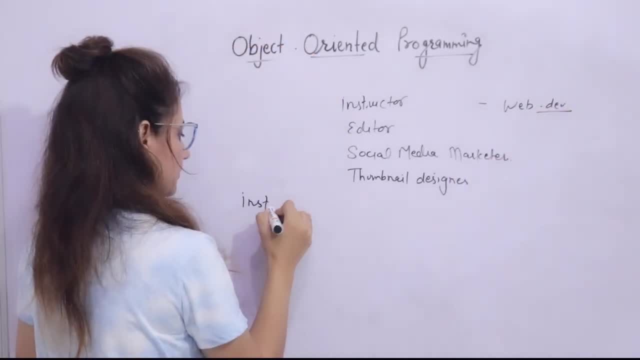 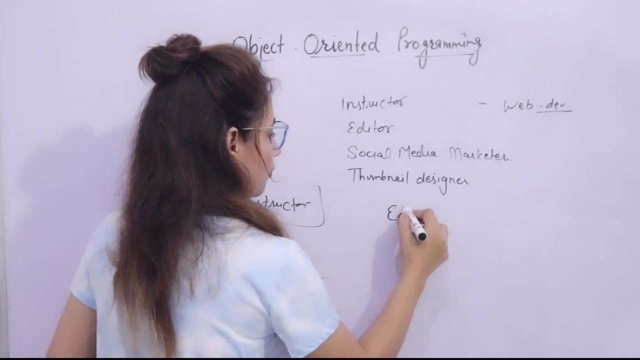 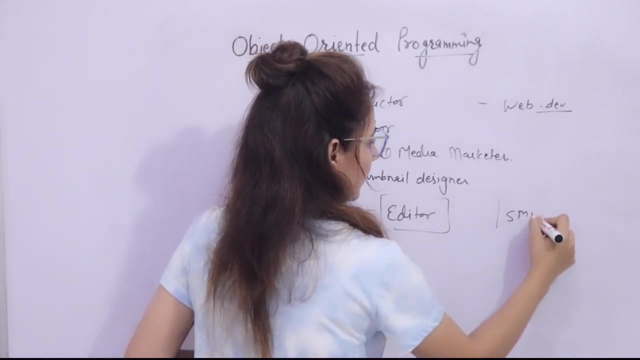 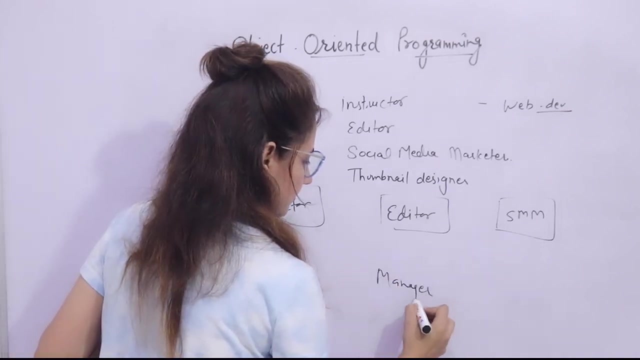 So I can hire one instructor that will teach this course right, And maybe one editor that will do the editing as well as thumbnail thumbnail- designing One. I will hire social media marketer and I would be like manager. right Now, my task is to manage these courses. 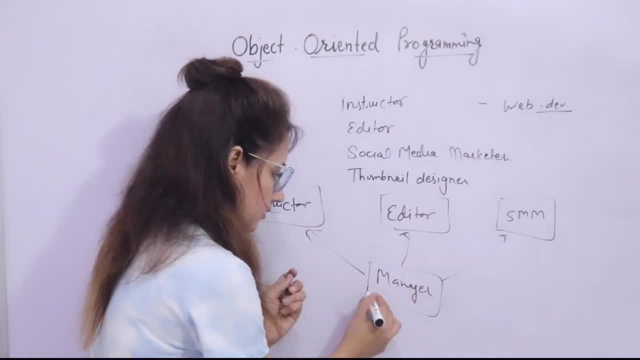 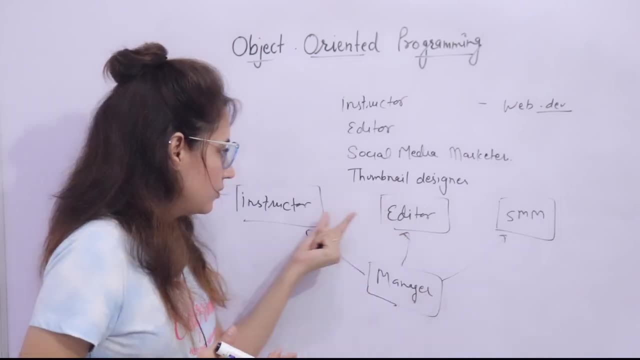 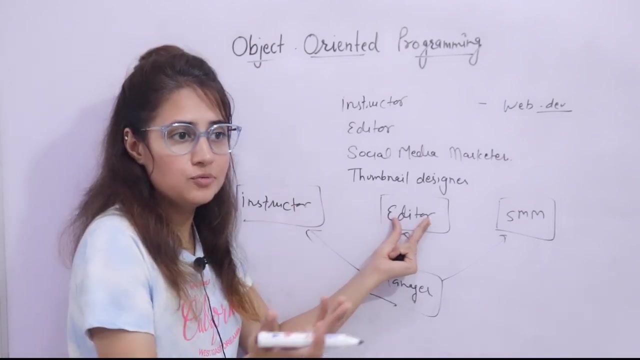 Now this manager, like suppose the manager is me. So I don't need to go in so much detail of how they are going to do their task. I don't need to tell how to teach to the instructor. I don't need to tell how to edit the videos, how to design thumbnail to an editor. 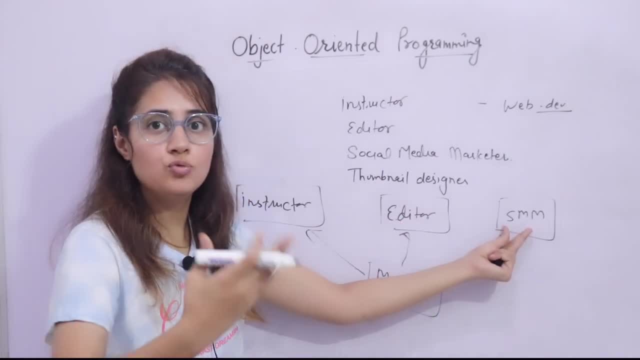 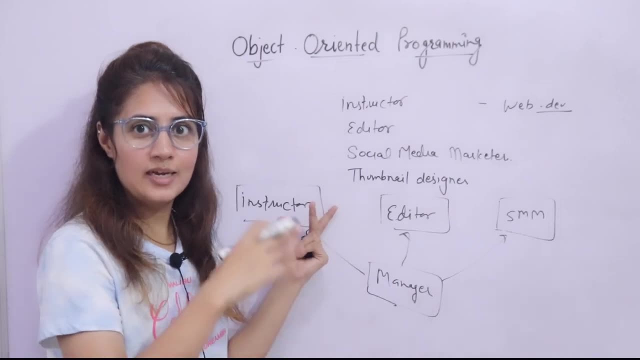 I don't need to tell a social media marketer how to do your job right. I don't need to worry about these things Because these are expert in their job. They know how to do their job better than me, I guess right. 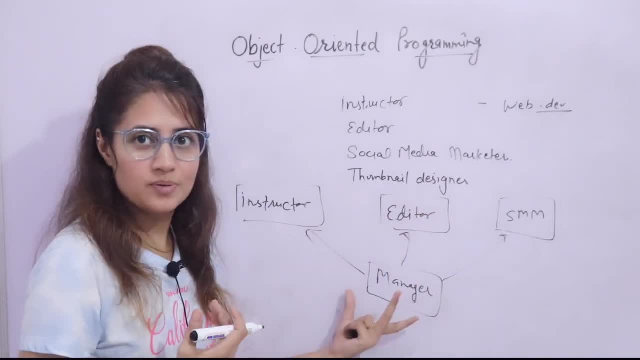 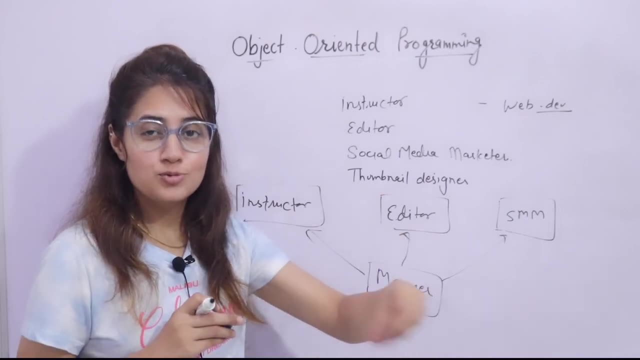 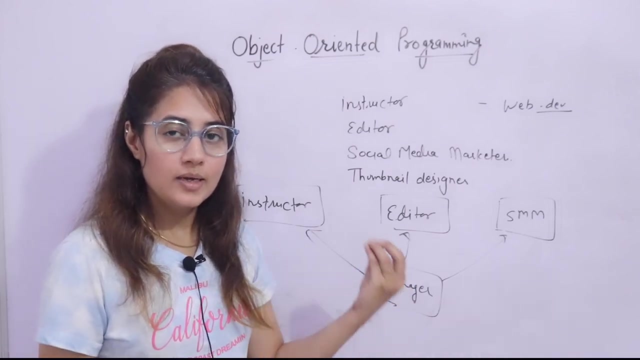 So this is going to simplify my task and simplify the relationship. So the same approach or the same concept we can use to simplify our code, to implement larger project, to make our project more scalable. the same approach, right, and see now one more. 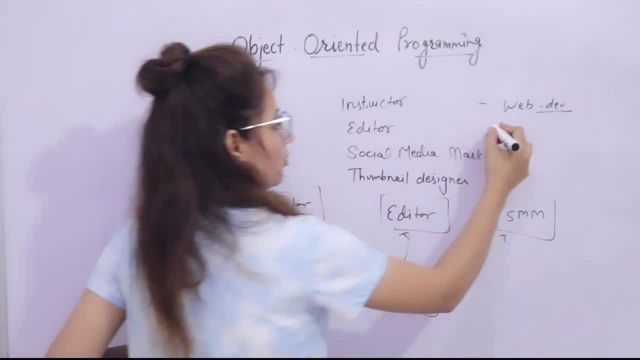 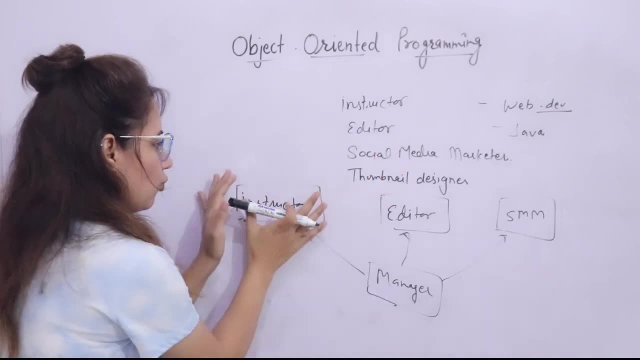 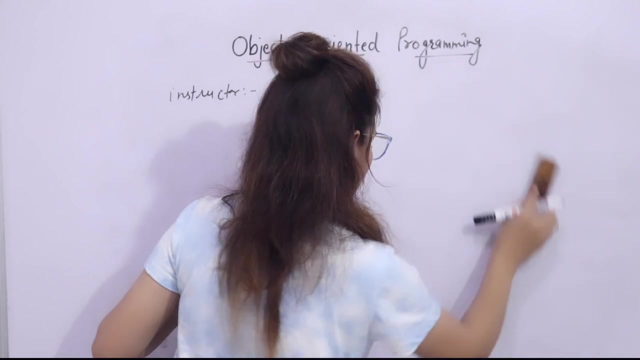 thing. So if I want to like start one more course about Java, so, or before that, let me just tell you something. Now let's take one thing, like I'm taking this instructor. So this instructor is having and see, as we know, object oriented programming, OOP is used. 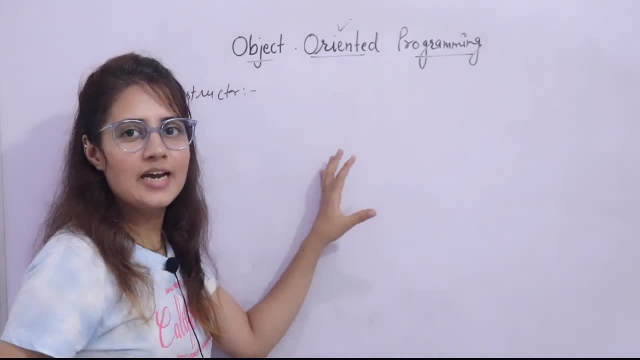 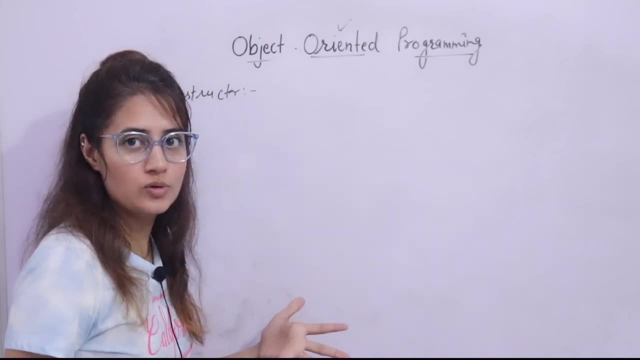 to model real world project, right? So let's create now a virtual YouTube channel. So let's create a virtual instructor, virtual editor, virtual social media marketer and everything, Okay, Okay. So let's do everything virtually, let's create right. 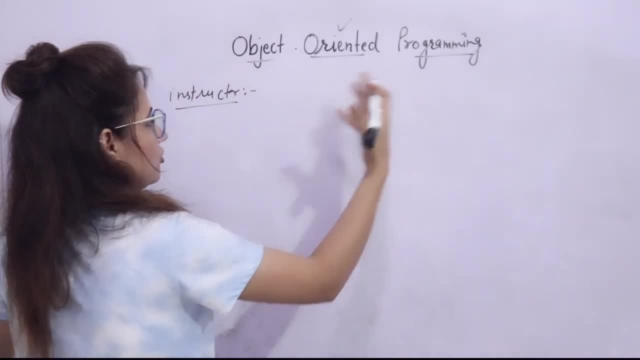 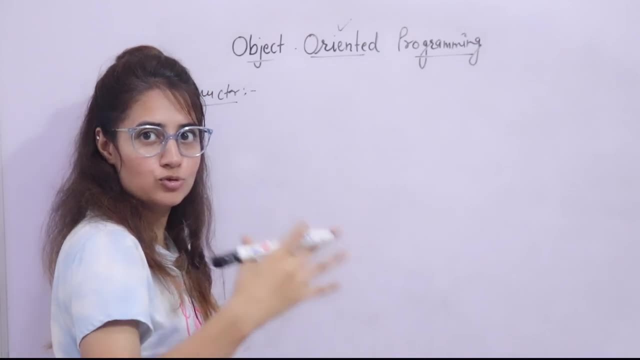 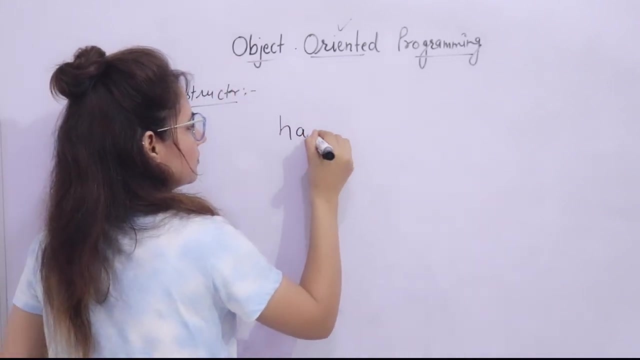 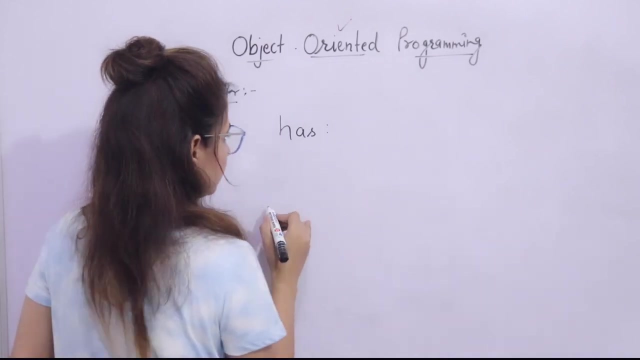 Now we need to model this, these things- instructor, editor and all in programming- right. We need to model these things in programming and, obviously, using OOP approach, we use, we model right Now this instructor. this is having some information right and it will do some tasks right. 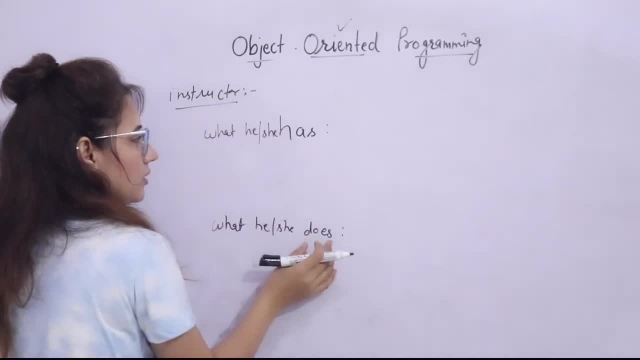 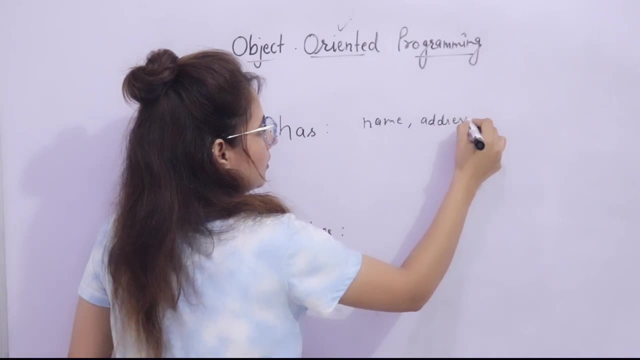 So two things: What, What he or she has or what he or she does. So it is having obviously some information, like name of the instructor, maybe address, phone number, and like some attribute, like has books, then we can say like true having. 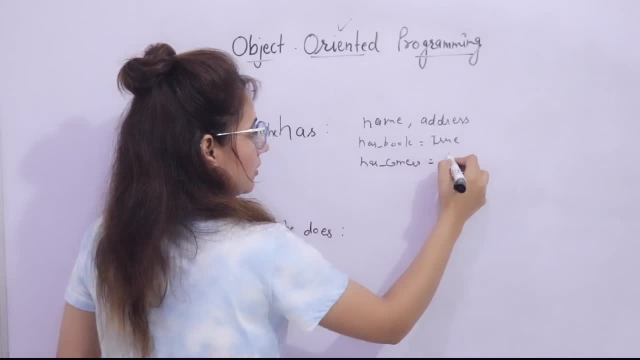 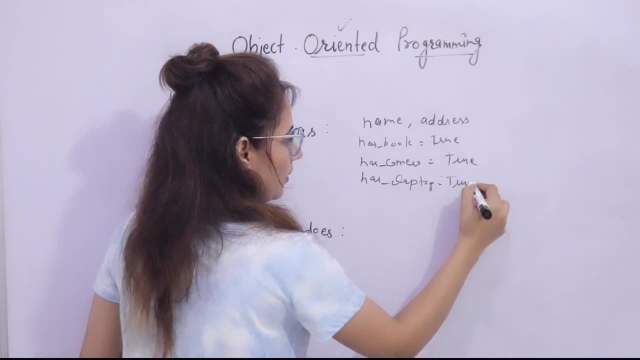 books, has camera, because to record the lecture we need camera- and, like, has laptop. that is also true, or maybe something is false. So it is having something, some information, right And it is having some information right, So it is having some information right. 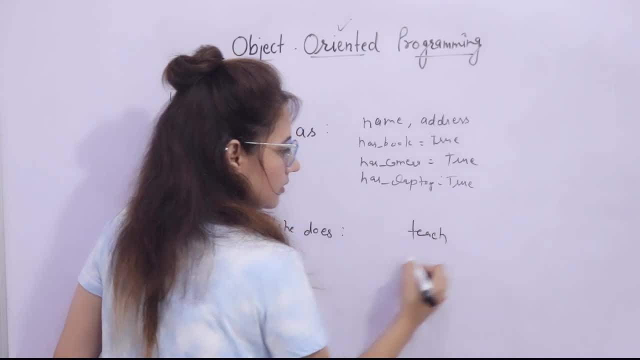 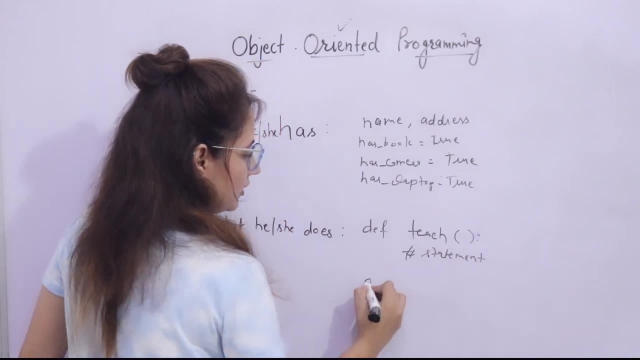 And it will do something. What it will do: Teach, Teach. So we can say like def, teach. we can define a function and here you can write down some statements and maybe other thing, other function we can do, like def, it will also prepare quiz. 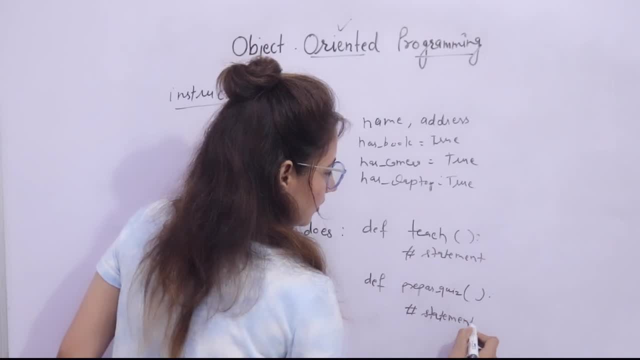 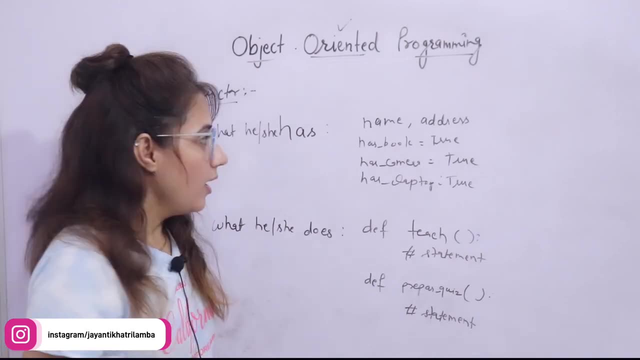 So that is other thing. So this is what it is having. this is what it will do right Now in programming terms. See, these are simply things. This is what it is having. This is what it will do. See, we know these are variables. 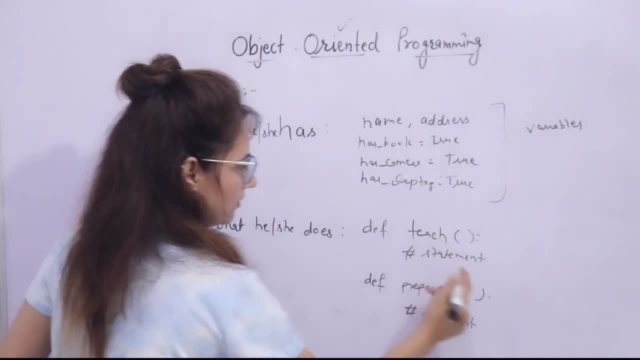 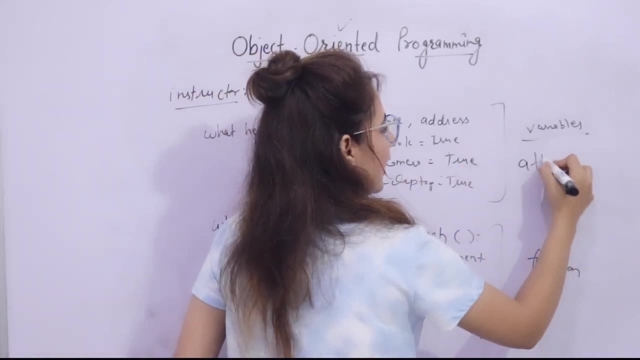 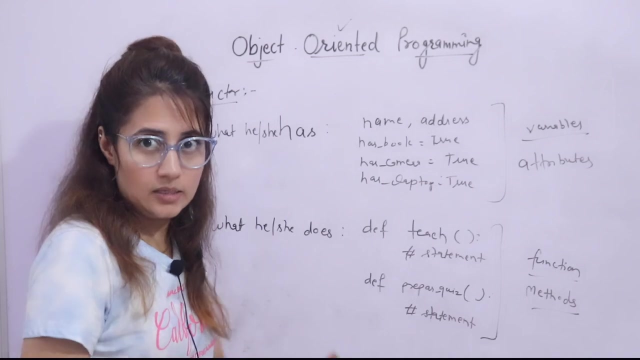 If simply I say because these are variables, obviously, and these are functions, but in case of object oriented programming, we call the variables as attributes and these are known as methods, not functions, methods. and there is some reason because, see, these variables and these functions are not free floating. 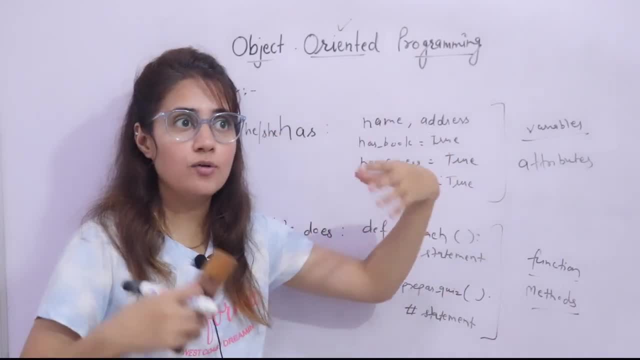 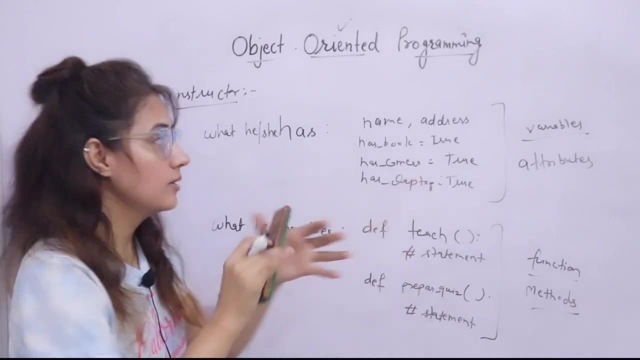 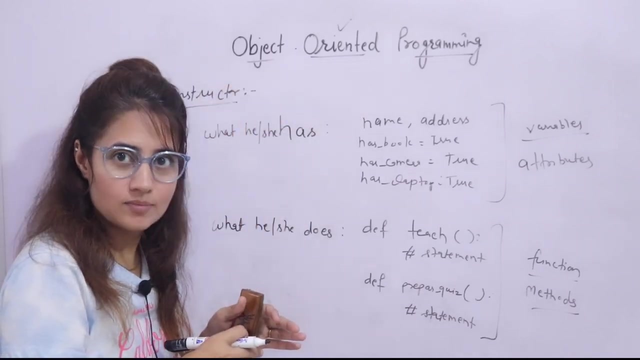 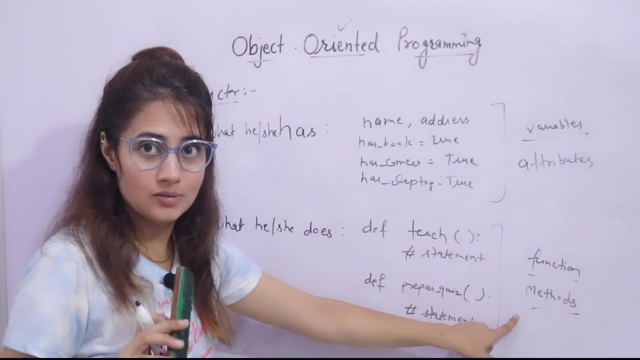 In PoP, the variables we take, like global data that was free floating, floating, move anywhere. These variables, these functions, are associated with an entity that is instructor. So these things are associated with this thing. Right, That is why these are known as not simple variables attributes, Not simple functions methods. Right, Because 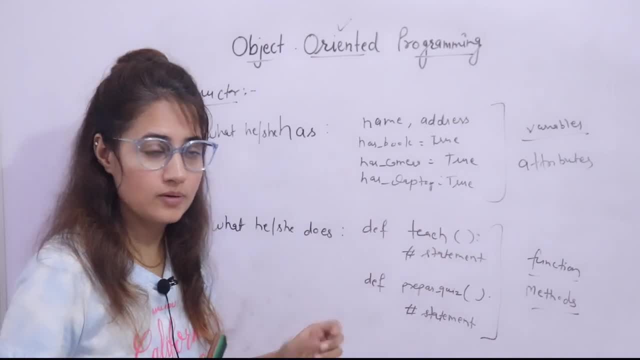 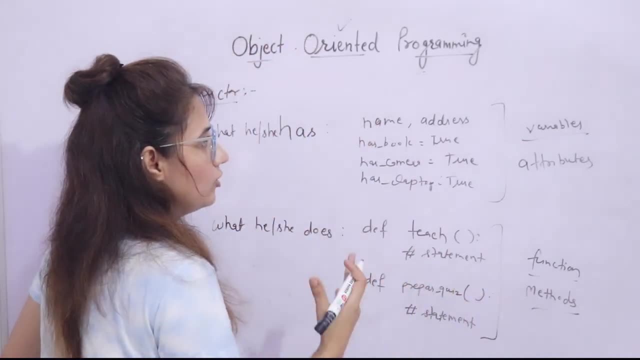 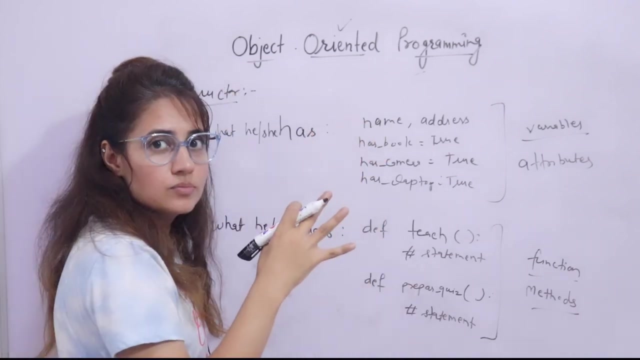 these are associated with something. These are not free floating in your program, Right? So in OOP we try to model real world object. So these object are having something, some information, these objects do something, So what they have, that thing is modeled with. 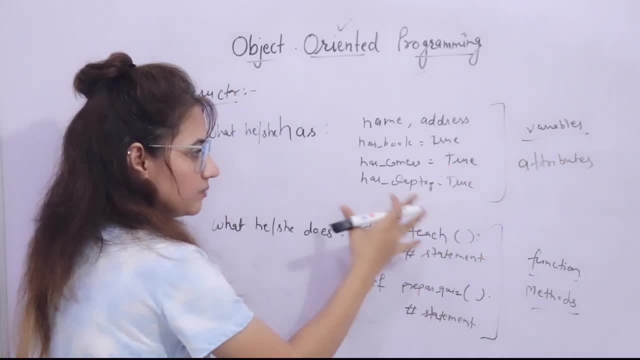 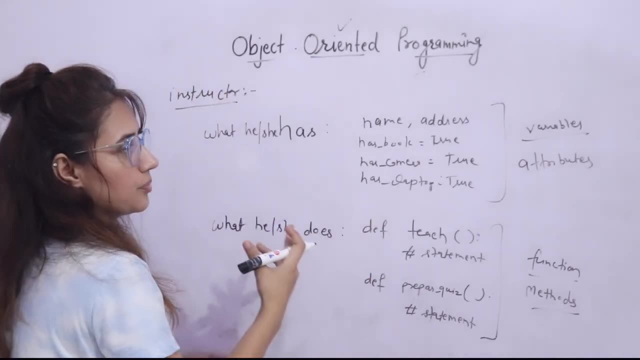 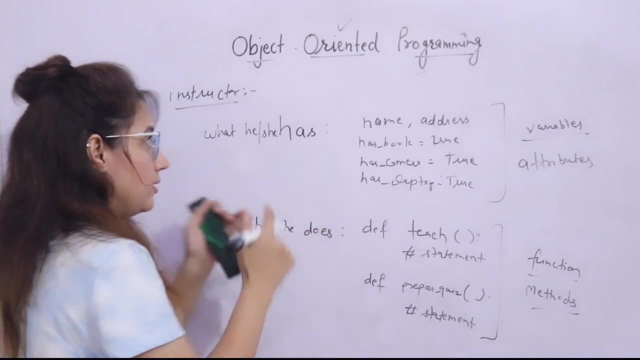 the help of attributes and what they do. that thing is modeled with help of methods, Right? So simply we can say: an object is just a way of combining some piece of data and some function functionality into a same thing, into same thing, like into a box. this is same thing in a box only. 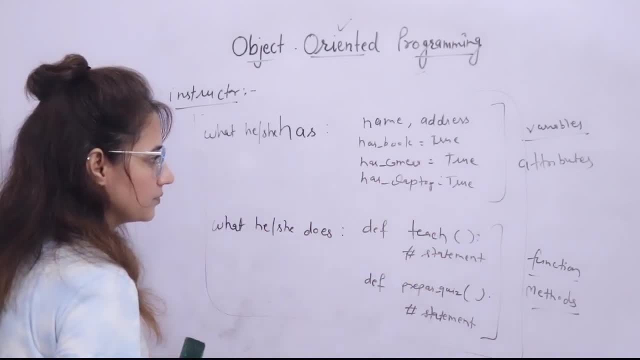 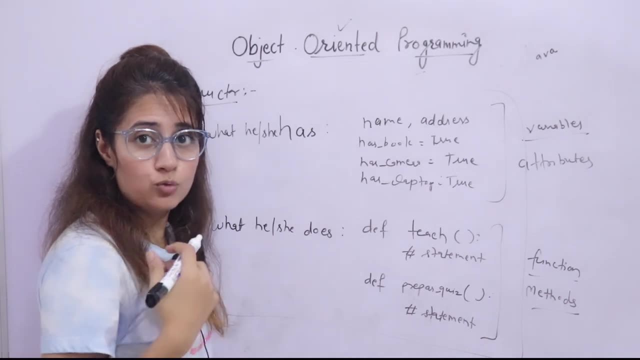 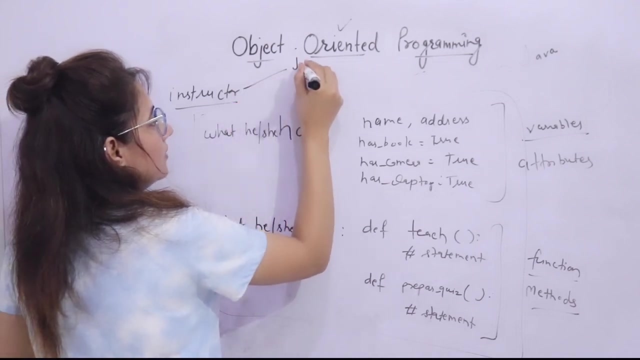 we are having this and this as well right now. if i want to start another course, like java, so i can hire one more instructor. if i want to start another course, i can hire one more instructor. that is fine, right, so, instructor, suppose i have hired, like jia, one more instructor. 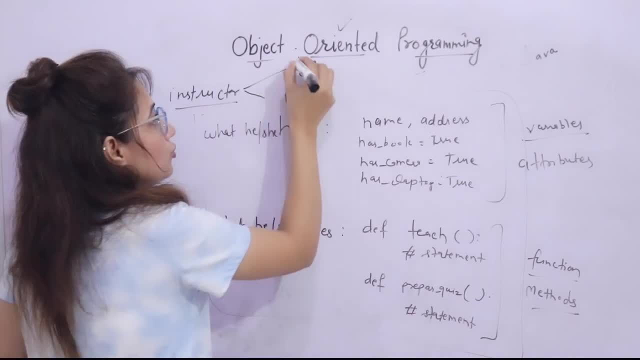 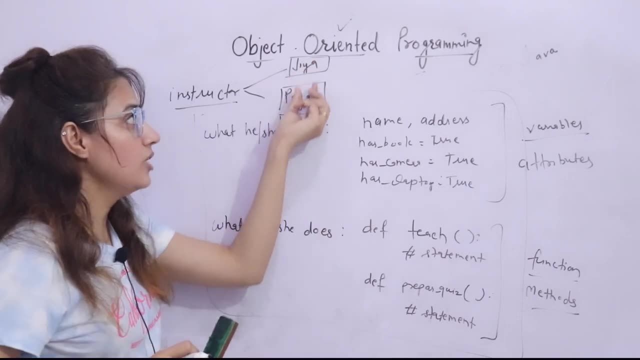 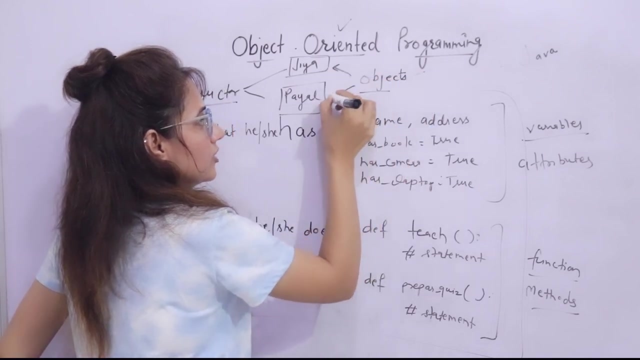 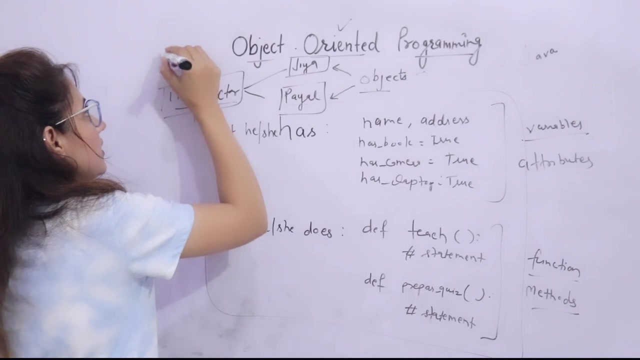 pile, maybe one more instructor. so now, see now these actual thing, these actual person jia pile. these are known as objects in object oriented programming. these are objects, right, and this, this instructor. this is simply a blueprint or a design. this is known as class. so class is simply a blueprint, just two. 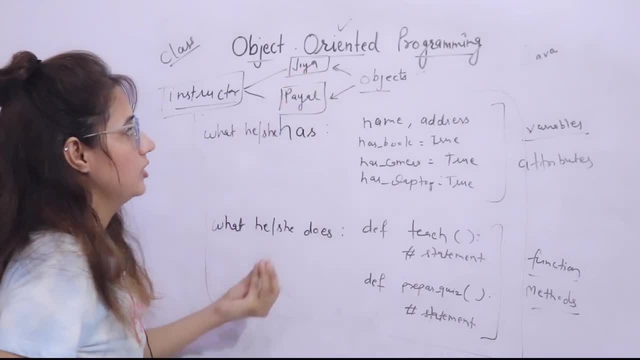 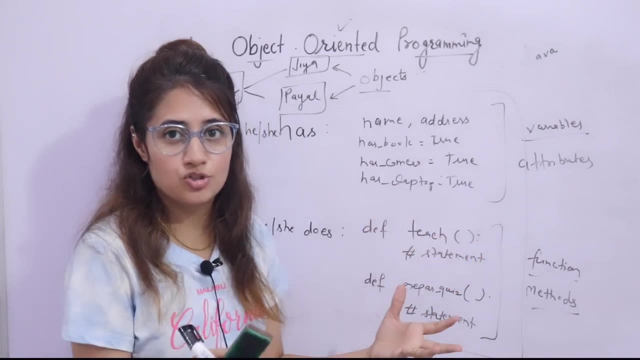 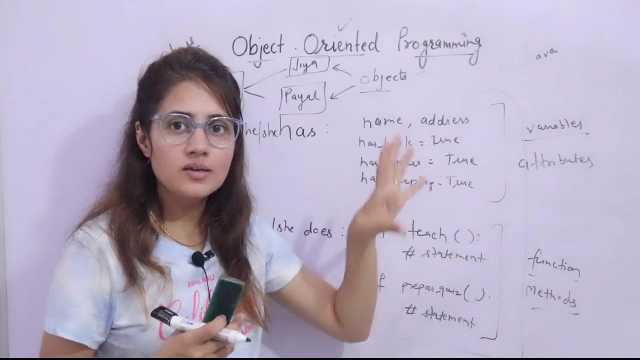 create objects. so these actual things, these are objects, right, like if you are going to build a house, then the map or the sketch of that house is what a blueprint, a design you have and using that design you can build a house. so that house says object and that. 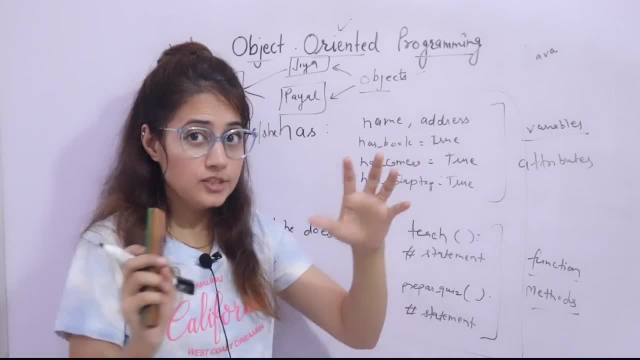 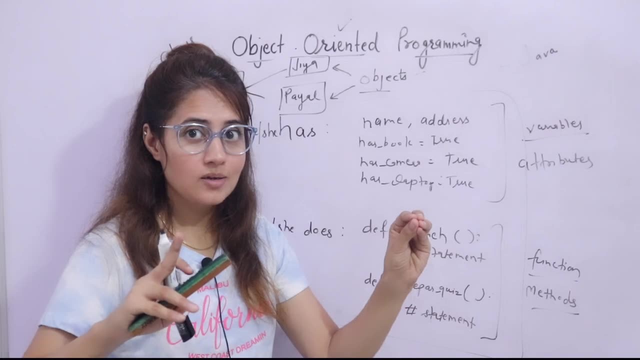 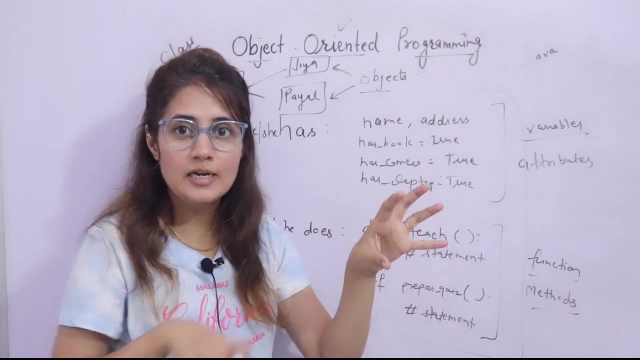 sketch or that map is what a class. and see, using that single map, we can, we can construct, we can design multiple houses. right, so we have only one class, we have only one design, we have only one blueprint. using that, we can build many, we can create, we can. 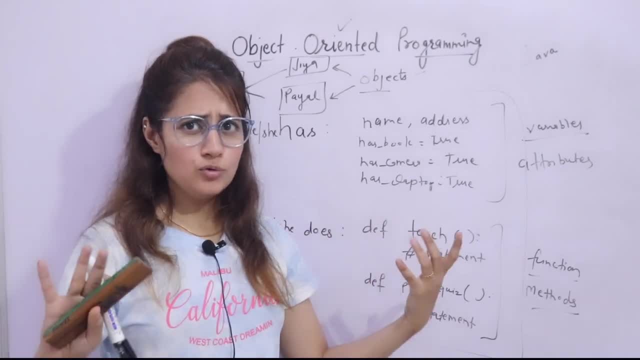 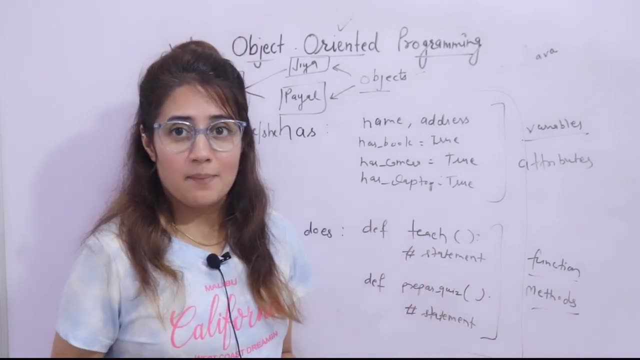 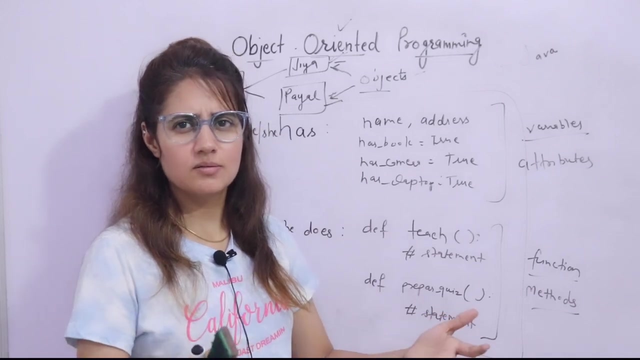 generate many objects right. so i hope you now you got the basic idea or an overview: what is a class, what is an object right and why basically we need object oriented programming right. so now the overview of object oriented programming, like basically why we need this right and what is.